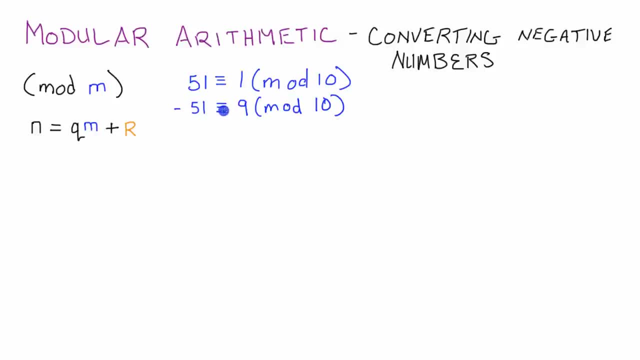 But, on the other hand, when we're dealing with negative 51, it's actually congruent to 9 mod 10.. So how exactly does that work? We want to go ahead and apply this formula that I outlined in the last video. 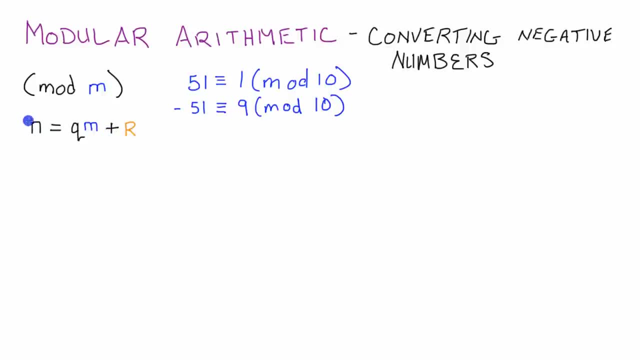 So let's go ahead and go through this step by step. So n represents the number that we would like to convert. In this case, n is negative 51. So we'll go ahead and write negative 51 here where n is, and then that's equal to q, which is just some number that's going to help us make the right-hand side equal to the left-hand side. 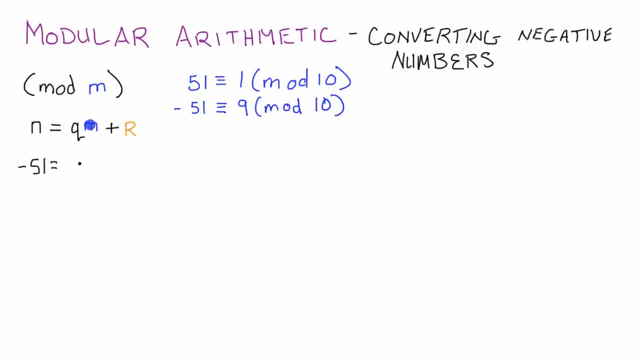 So we'll just ignore q for a moment, and then we'll go ahead and write our mx. So we'll go ahead and write our n here, which is our mod- In this case it's 10, and then we're going to add some sort of remainder here. 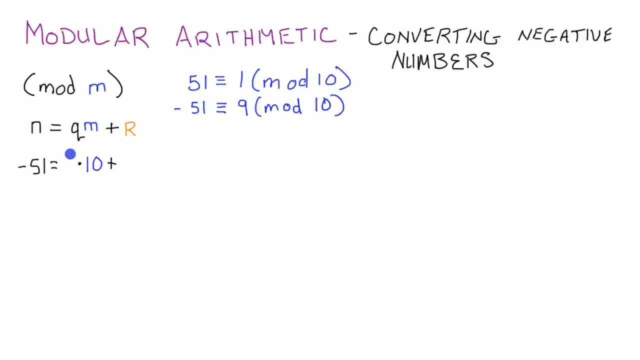 The idea here is we want to choose a q so that this portion, right here, the q times m portion, is more negative than the original number. If we chose a q of negative 5, negative 5 times 10 would be negative 50, but negative 51 is still more negative than negative 50. 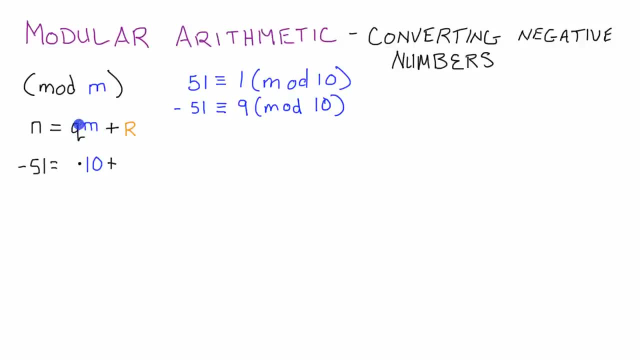 So we'd need to choose a slightly more negative q. If we chose a q of negative 5, let's choose negative 6.. So by choosing negative 6, we end up with the q times m portion being more negative than the number we're trying to convert. 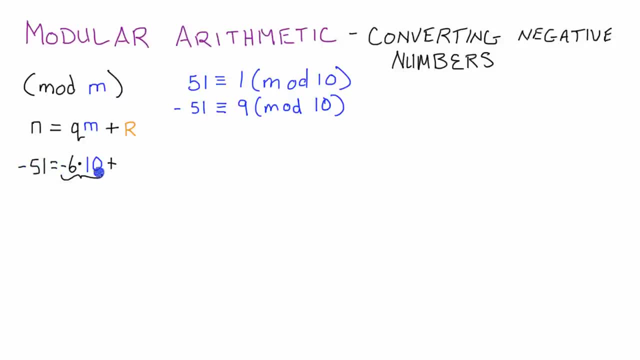 So we have: negative 51 is equal to negative 60, plus some positive remainder. So that's the trick right here: choosing a q so that it's just slightly more negative than the number we're trying to convert. Now we wouldn't want to choose q as a negative 7, because that would put 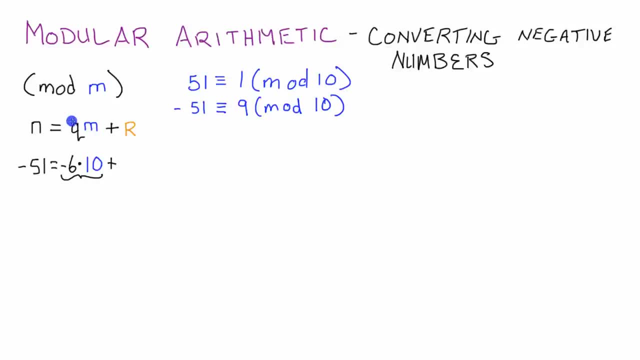 that would push us too far and our remainder would be outside of our mod. We want to find the first q, the first integer, that we can multiply by our mod to make us more negative than the original number. So we have negative 60 plus some number equals minus 51.. 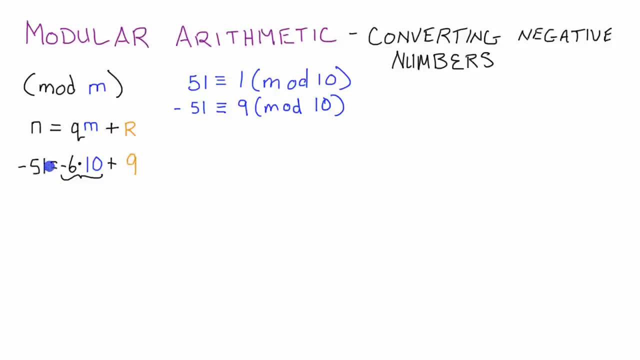 So it turns out that that remainder is 9 in this case. So what we end up having here- we basically have negative 60 plus 9- brings us back to negative 51. So therefore, negative 51 is equivalent to the number 9 when we're dealing with mod 10.. 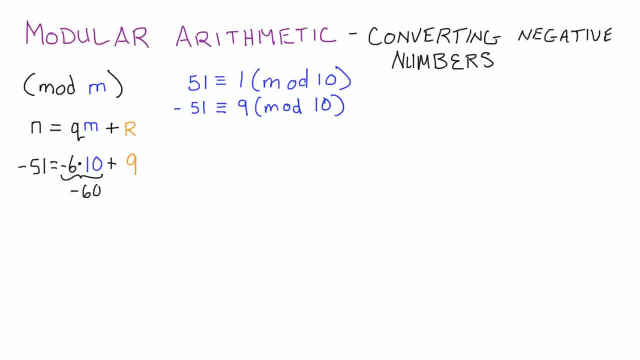 So that's how we get this relationship between negative 51 and 9.. So let's try this with another example. now Let's look at negative 37 and let's figure out what negative 37 converts to when we're dealing with mod 5.. 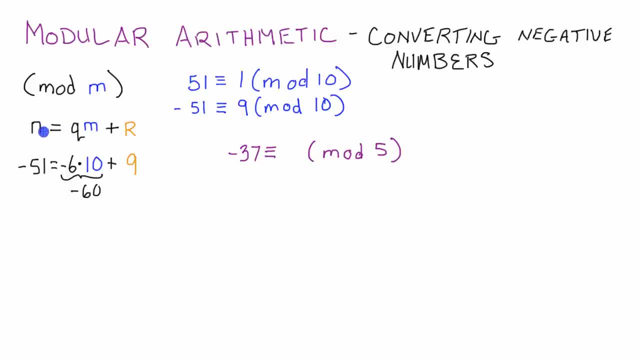 So we're going to take the same approach here and in this case is going to be the number. we're starting with negative 37. So we have negative 37 is equal to something, and that's something would be the q here that we're going to choose in a moment, multiplied by our mod. 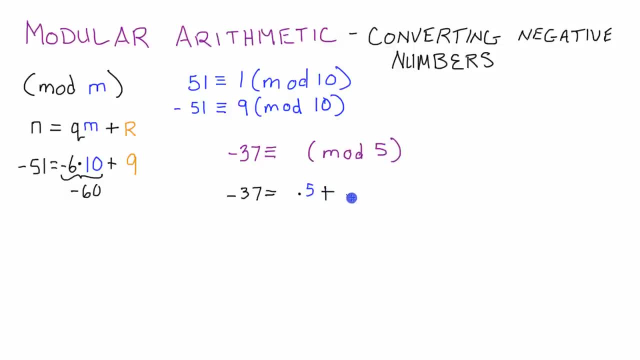 In this case our mod is 5 and then we're going to go ahead and add that remainder. So the idea here once again is we're trying to find the first negative integer that produces some sort of q times m that is less than negative 37.. 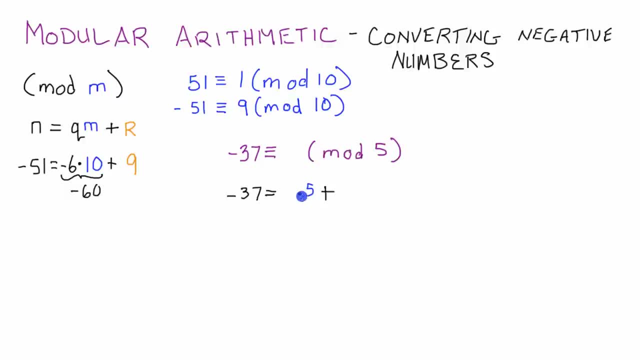 If we think about this, if we chose negative 4, negative 4 times 5 is negative 20.. We're not quite less than negative 37. Negative 5 times 5 would give us negative 25, we're still not there. 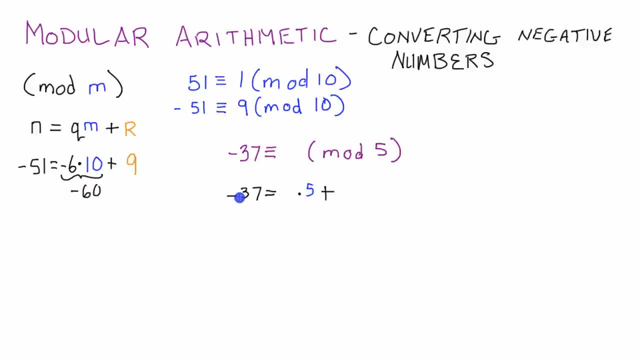 Negative 6 times 5 would give us negative 30,. we're still not there. Negative 7 gives us negative 7 times 5, which would bring us to negative 35. We're getting pretty close. and then when we go to negative 8, negative 8 times 5 will give us negative 40,, which is finally less than our negative 37 here. 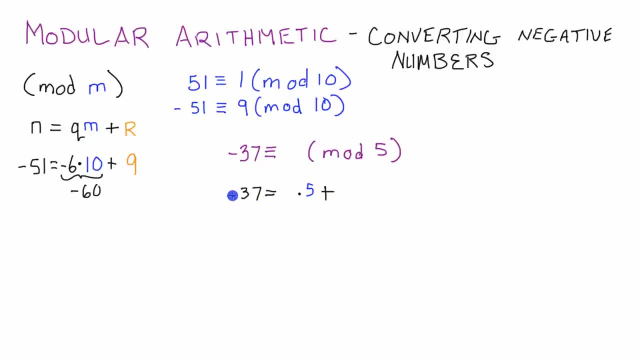 So when we get to that first number that puts us below negative 37,, that's the one we want to keep. So, in this case, negative 5, negative 6,, negative 7, and we just kept on going down the list until finally we got to negative 8,, which put us below our negative 37. 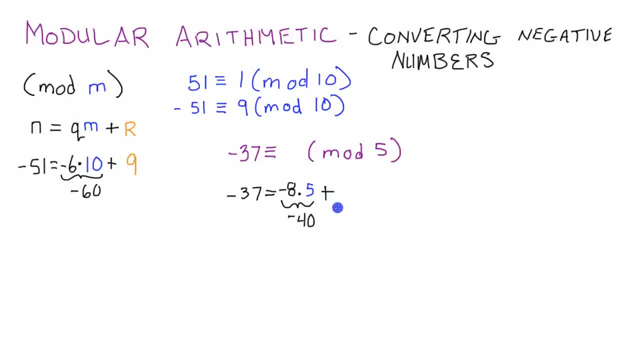 Negative 8 times 5 is negative 40, and then the idea is, the remainder is going to be some number that's within the mod. that essentially brings this number back up to the original number we started with. So negative 40, and then if we back up or add 3 to it, then we create a true statement once again. 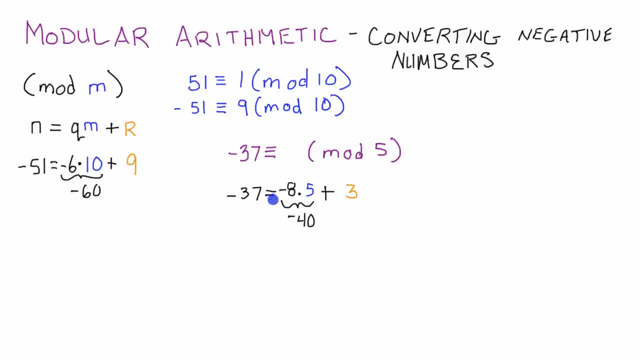 So negative 37, we can say is congruent to 3, mod 5.. We'll go ahead and write that down here. So if we end up with a negative 37 when we're doing our cryptography, we can convert that to a positive 3 if we're dealing with mod 5.. 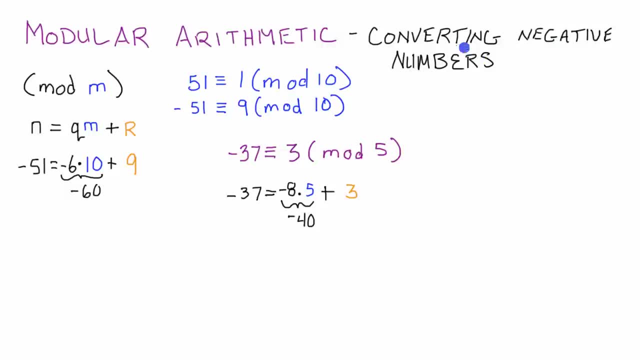 So, anyway, that's a good introduction to converting negative integers so that we can use them within a particular mod. Thank you guys for watching. stay tuned for more cryptography videos. have an excellent day and, if you haven't already, don't forget to subscribe. Subtitles by the Amaraorg community. 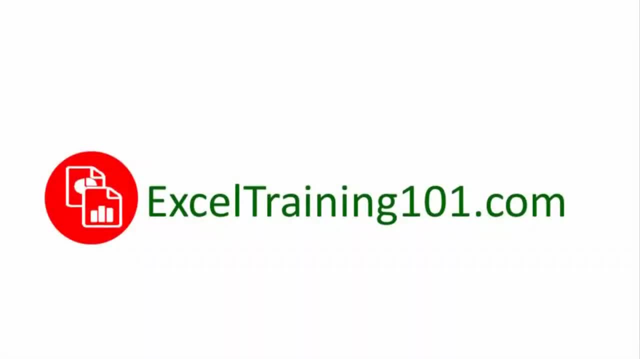 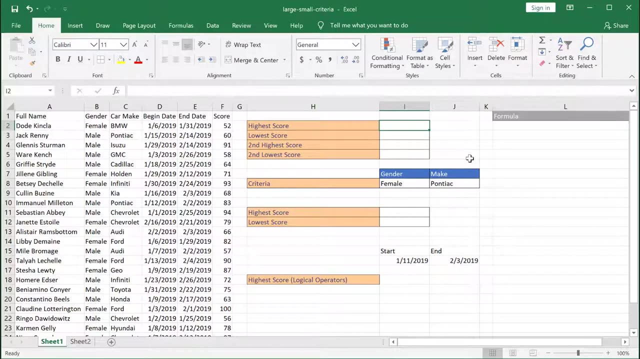 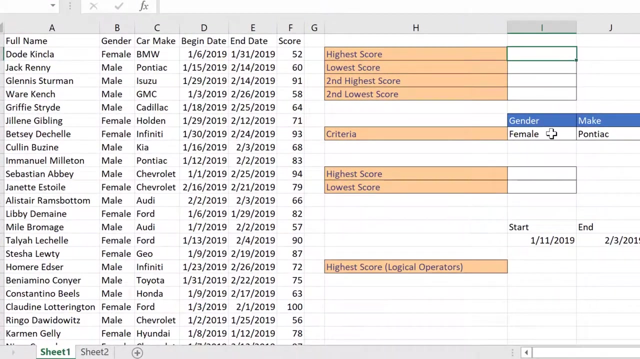 Hi, In this video I'll show you how to find the largest and smallest values based on a criteria. I've got some options here. We're going to look for highest and lowest scores and the second highest and lowest scores. That's another example, And if we've got some, 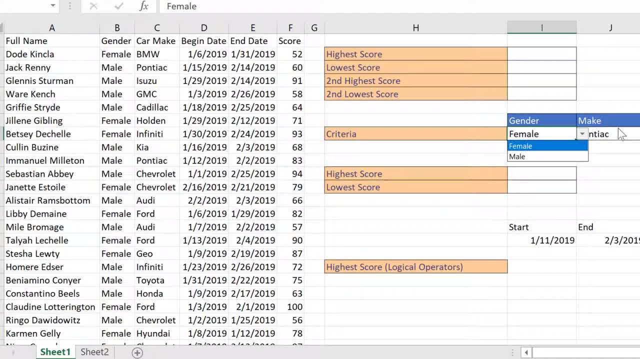 other criteria that are more specific. let's say we have this drop-down for male, female and this drop-down for the make of the car And those. we can use that to have inputs into our high and low scores based on these various parameters or criteria, If you're. 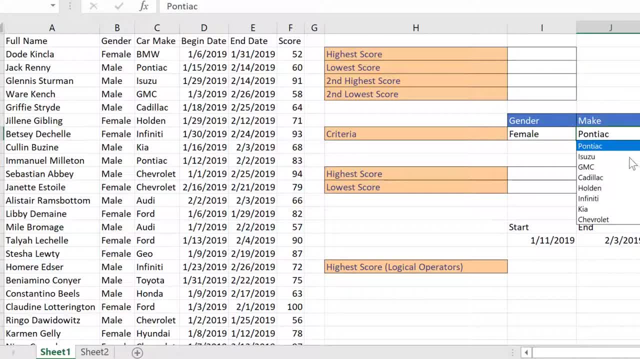 interested. at the end of the video I'll cover how to create these drop-downs. So that would be something maybe later at the end. But see, with this we can use the criteria here, And in addition to those criteria we can also use logical operators. the greater 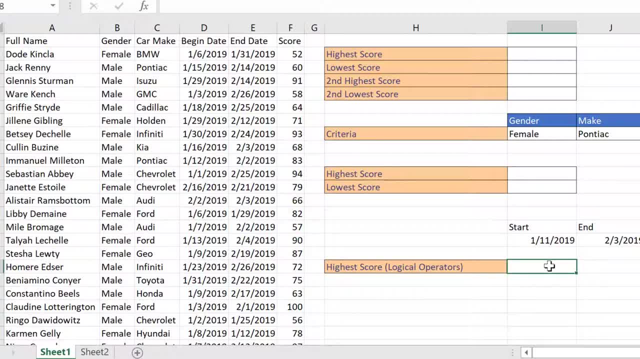 than or less than, And I'll show that over here in this section. So let's start off with the highest score. So the highest score. if you're already familiar, you can use the max function. The max function. let me tab that. I'll look for all the scores here. 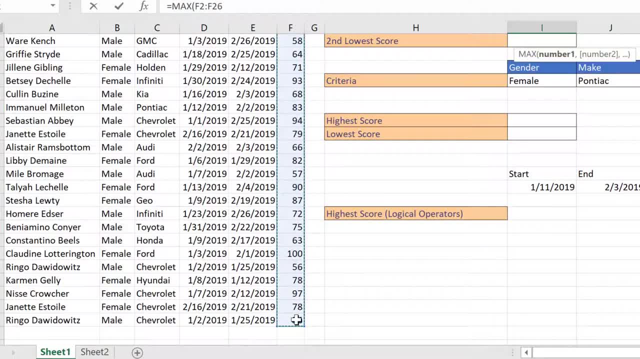 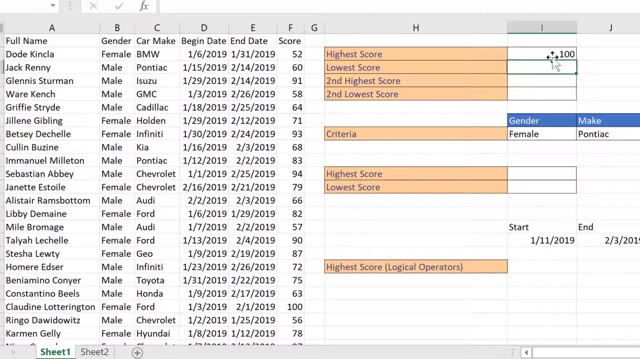 Let's see F2 to F26.. Press enter And we have our high score, which is 100, right here. That's the highest score. Now all I need to do is just bring that control C to copy, control V to paste. And one thing you'll notice too, if I didn't set my absolute cell reference. 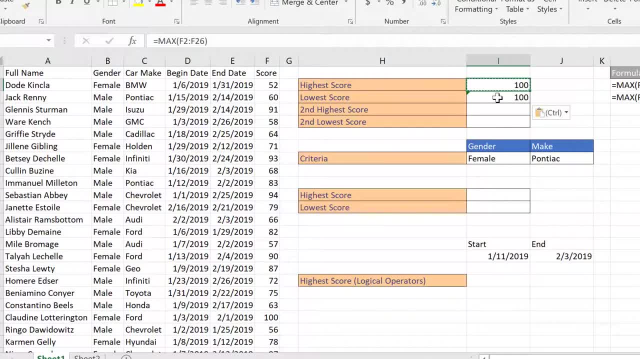 meaning that I didn't have the dollar number. I'm going to have the dollar number And I'm going to have the dollar signs in front of the F2, F6. When I copy that down, it offset it F3 to F27. So that's what happens when you copy it. So press the F4 key here to put.